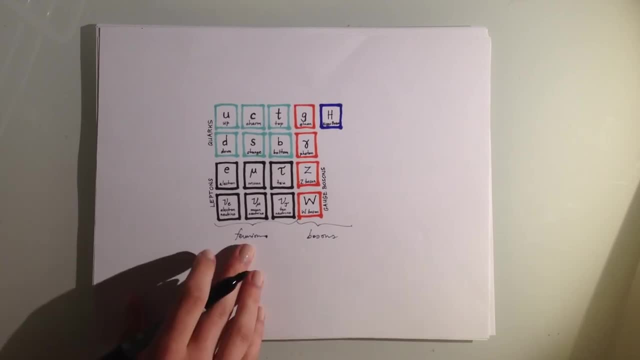 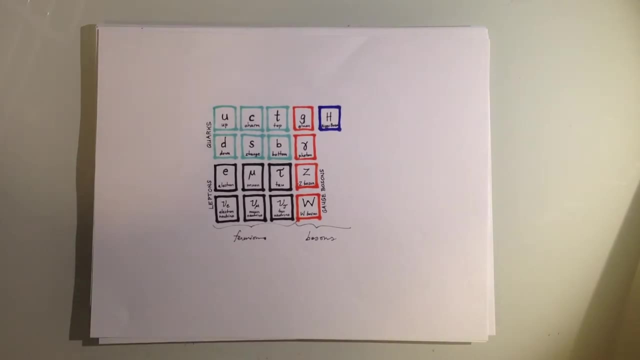 is that it can be broken down into two main groups. On the left, you have the fermions which make up matter, And on the right, you have the bosons which carry forces, Though you probably can't tell from this picture. 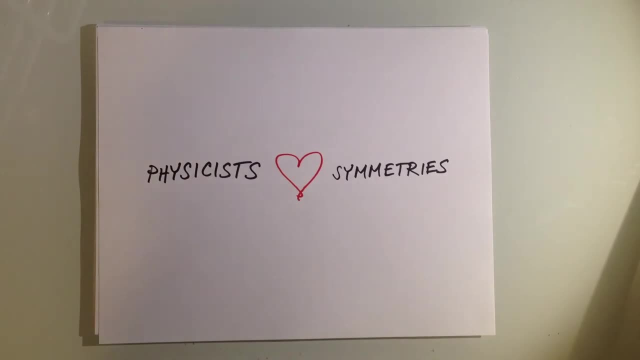 the standard model has a ton of symmetries. It's one of the reasons physicists like it so much. Physicists love symmetries. These symmetries help to answer a lot of questions about how particle physics works, But we still have a few nagging questions. 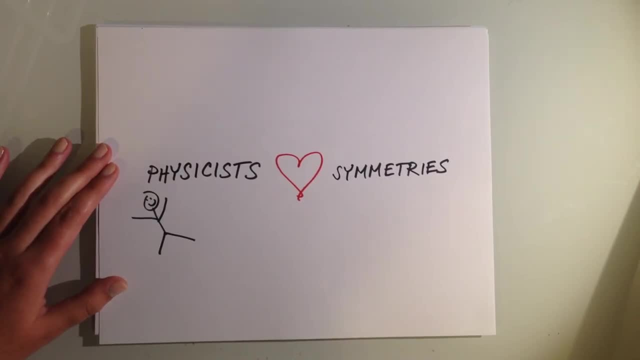 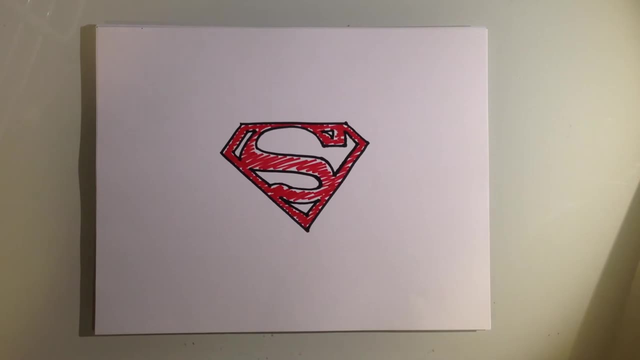 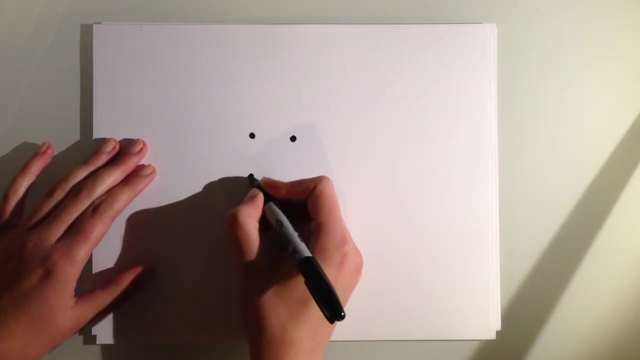 that the standard model just can't answer. So what do we do? Introduce a new symmetry. And what should we call it Super symmetry, because it's super. If we go back to our original square, I can show you how I like to think about it. 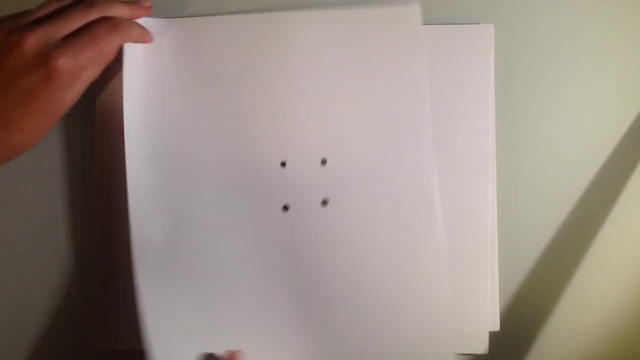 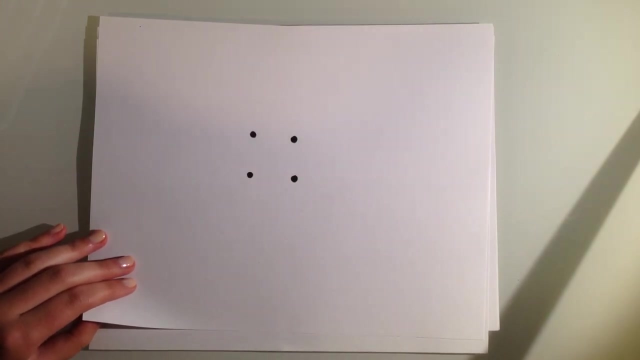 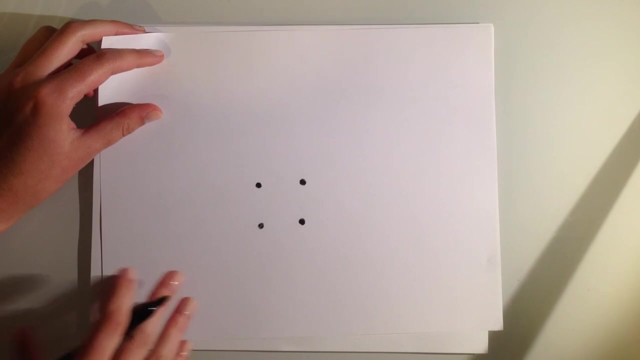 This square and the rotations and reflections we did before represent the standard model. By introducing super symmetry, we effectively double the standard model. It's kind of like doing this. See, we have another invariance. The Sharpie has bled through, so I. 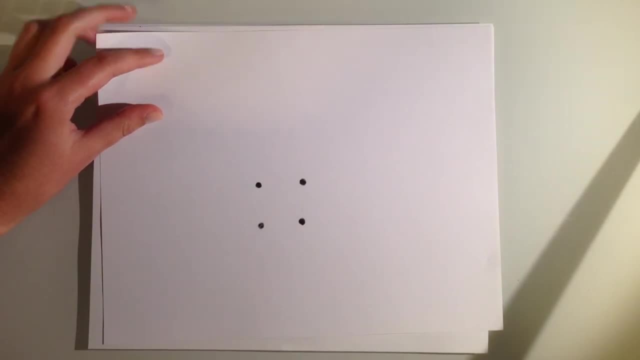 can flip the whole page over and still get a square. The actual idea behind super symmetry isn't too hard to follow either, although understanding the motivation is a bit more complicated. The idea is that for every fermion, remember the fermions, the guys who make up matter. 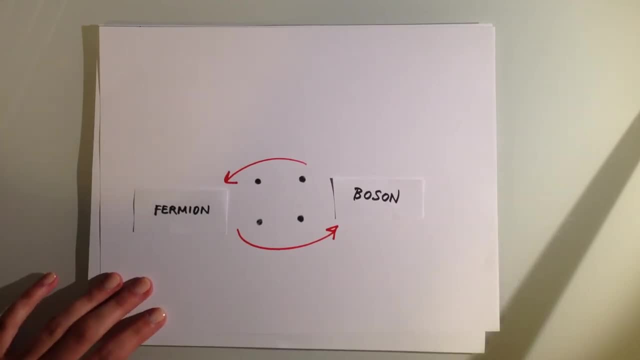 And the bosons are the ones who carry forces. OK, so for every fermion there is a boson counterpart, And for every boson there is a fermion counterpart. By requiring this, we double the amount of particles that there should be. 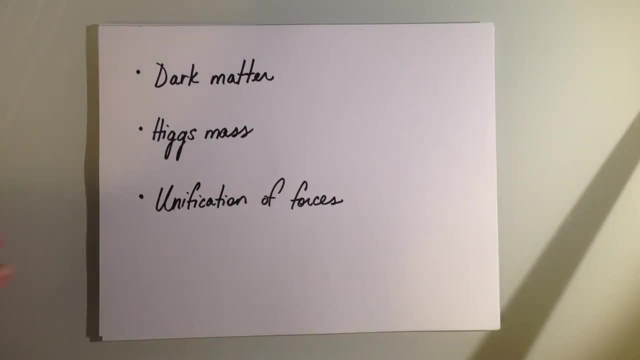 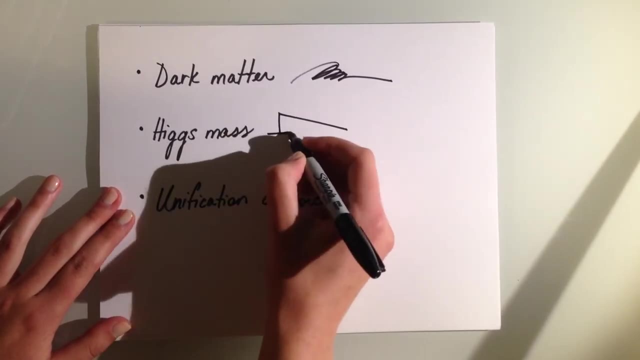 The reason this is an idea that physicists like is because it helps to answer a lot of questions. It helps to answer a lot of questions we still have about the universe, including what dark matter might be, why the Higgs boson, the particle that gives stuff. 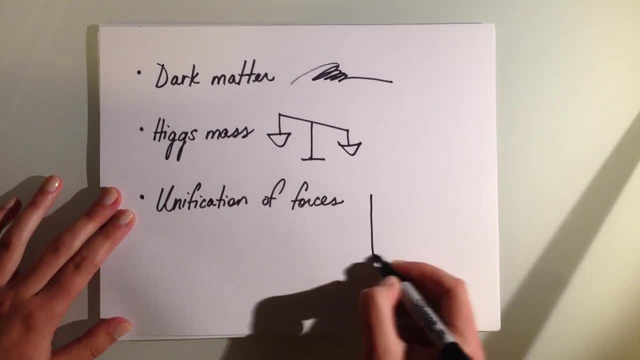 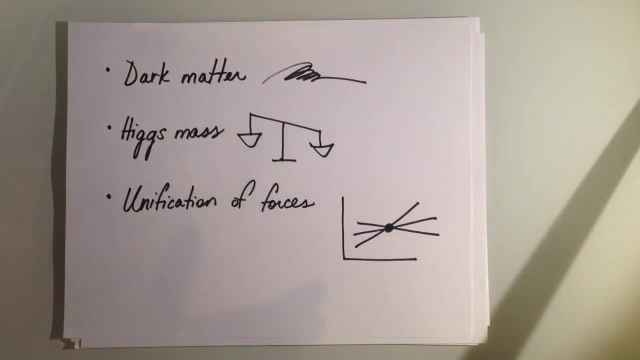 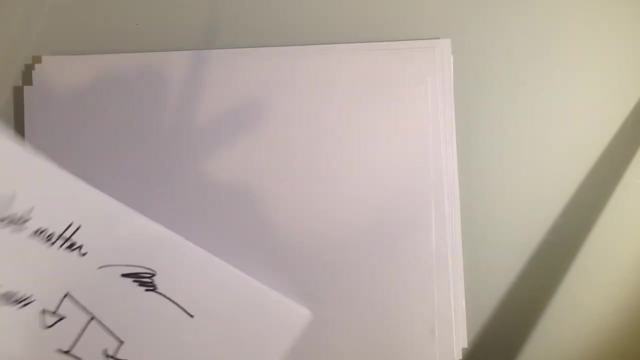 mass is so light and how the different forces could have all been bundled together in the early universe. It sounds pretty great, right? So how come it's just a theory? Why haven't we seen any supersymmetric particles? The issue is that we expect supersymmetric particles. to be pretty heavy, which in particle physics means they're hard to see. We try to find them by smashing other particles together near the speed of light and seeing what is spewed out in these collisions, But up until now we haven't had enough energy.